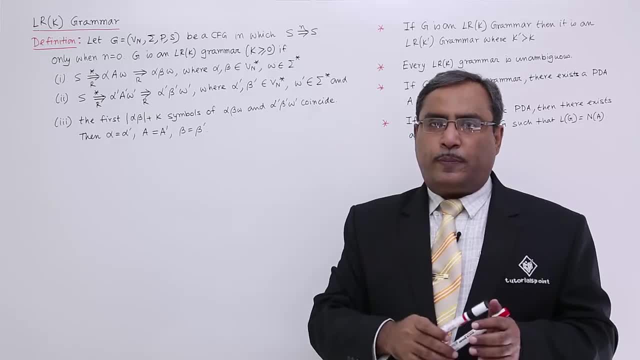 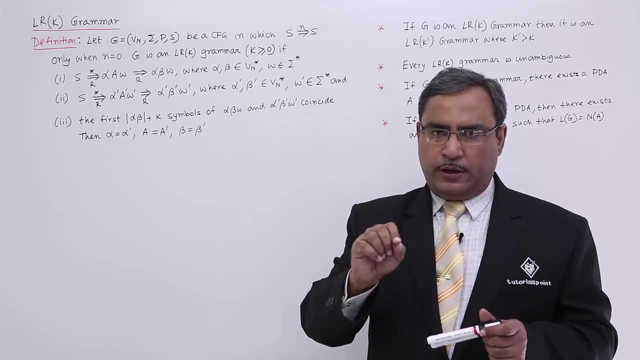 denotes in the input string: we shall read K number of characters at a time. So this is LRK. So L means I shall read K number of characters at a time. So this is LRK. I shall be reading the input string from left to right. R means rightmost derivations. 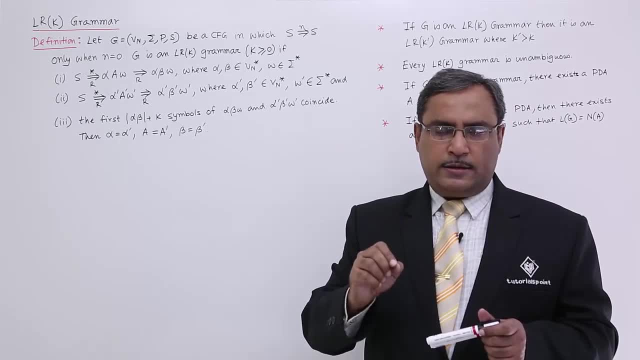 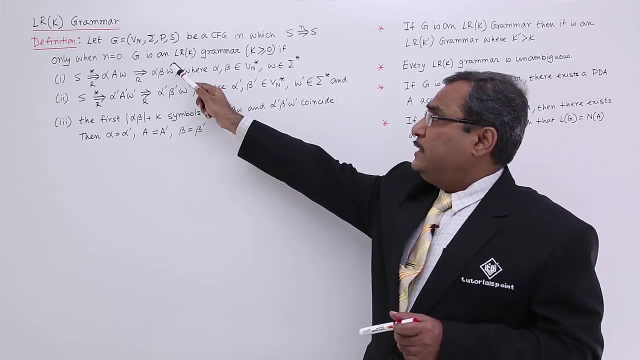 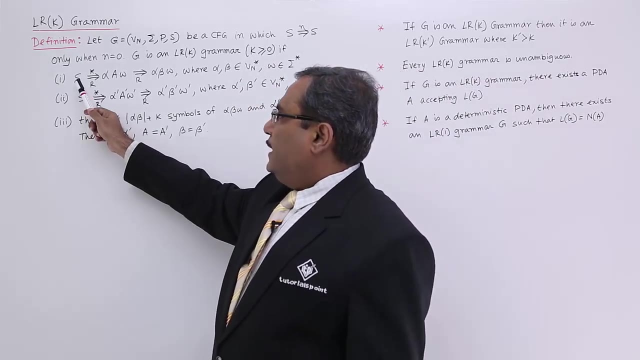 will be used in the sentential form, and K means we shall read K number of symbols from the input string. okay, So a G is an LRK grammar, if, and only if. So all these three conditions are to be satisfied. okay, What is the first condition? S from the rightmost. 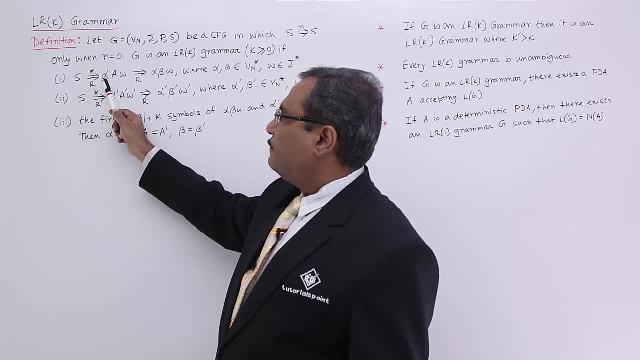 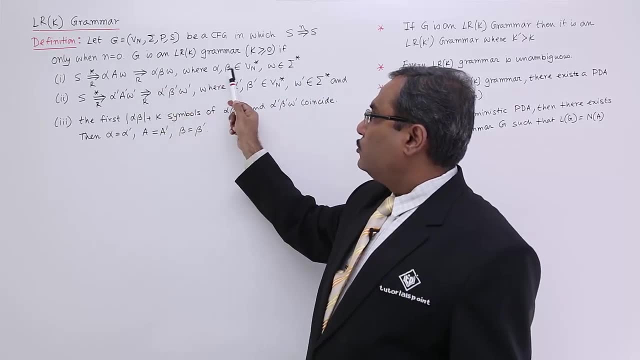 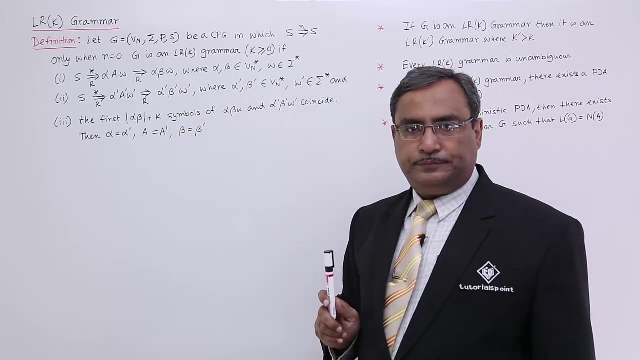 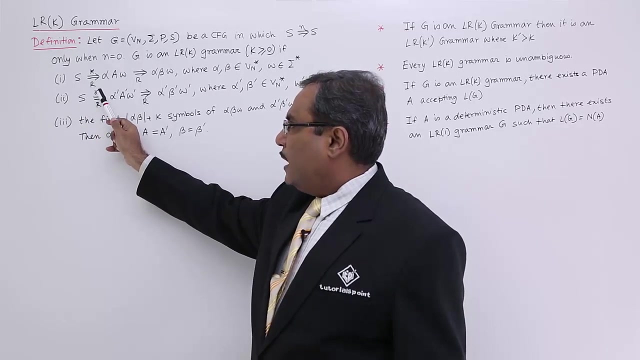 derivation using multiple time production rule. I am reaching to alpha AW. Then I am reaching to alpha beta W, where alpha beta belongs to VN star. That means that they are simply non-terminals and W belongs to sigma star. okay, Second case: from S, from the same start, symbol S, using rightmost derivation, after applying: 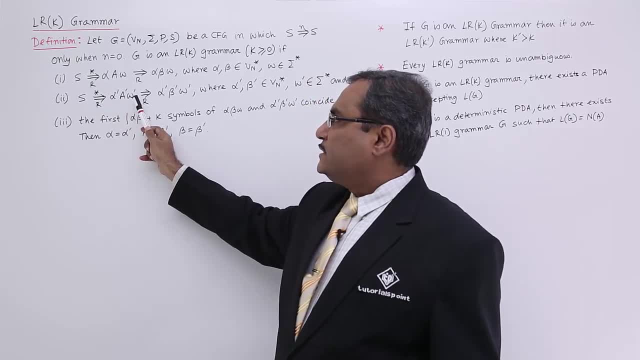 multiple time production rules. I am getting alpha dash, A dash, W dash, then rightmost derivation, I shall. I am going for alpha dash, beta dash and K. So Al再見 is valorizing the output, meaning that at the same time I am going for alpha dash and W dash. 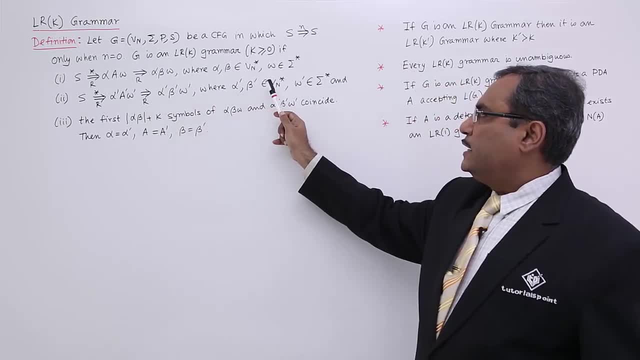 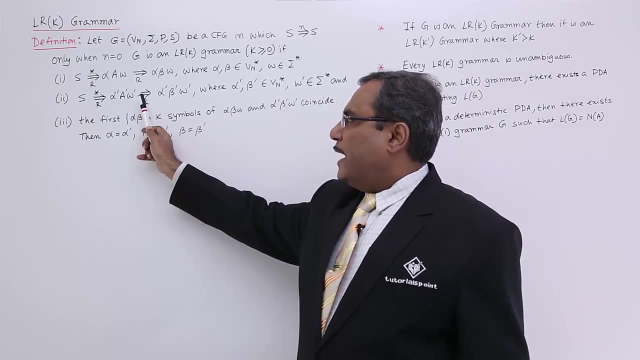 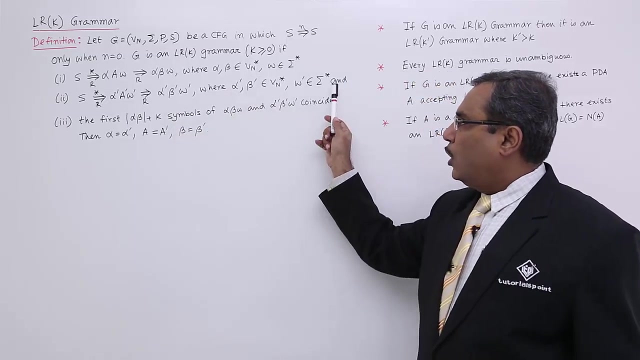 W dash. So now, where alpha dash and beta dash belongs to Vn star and W dash belongs to sigma star, Now you see, in case of rightmost derivation I am getting A. only that is the non-terminal, So that has to be deduced. So now, in this way it has been obtained. So that is my condition number 2. 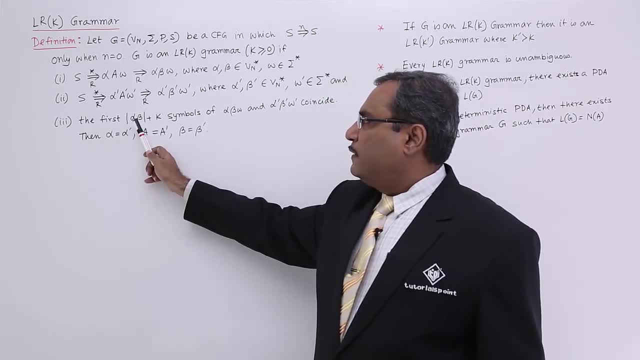 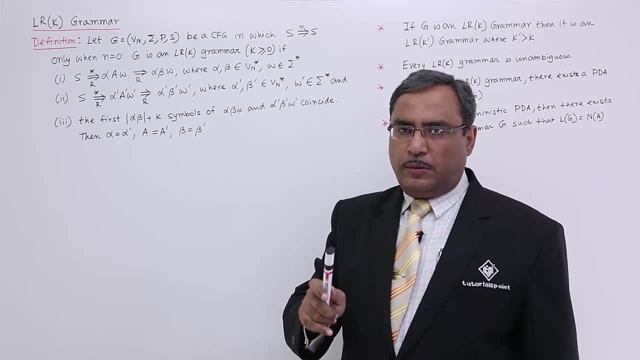 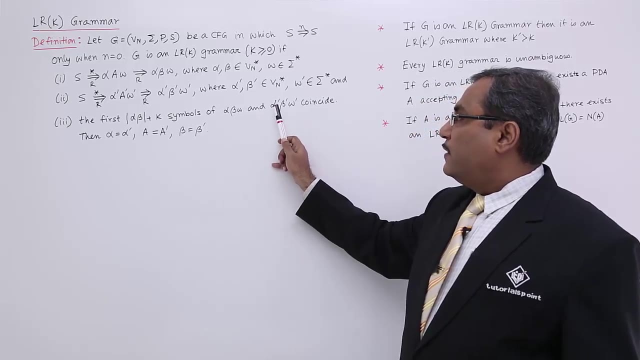 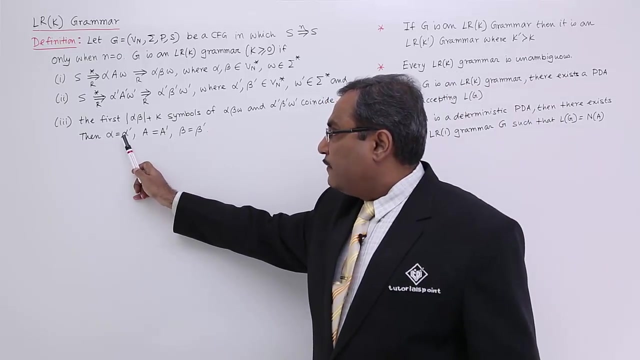 and condition number 3 is that the first alpha beta mod means length of alpha beta. That means number of non-terminals in alpha plus number of non-terminals in beta plus k, number of symbols of alpha beta, W and alpha dash, beta, dash, W, dash coincide, That means then alpha is equal to alpha. 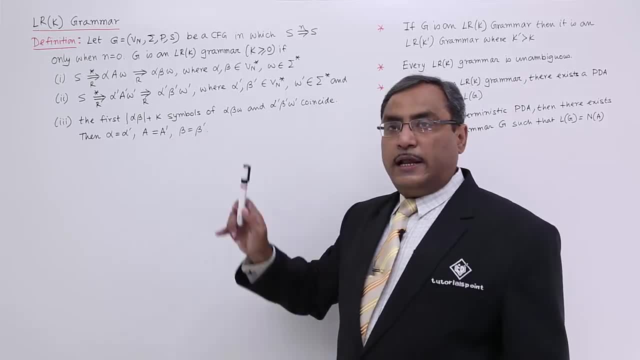 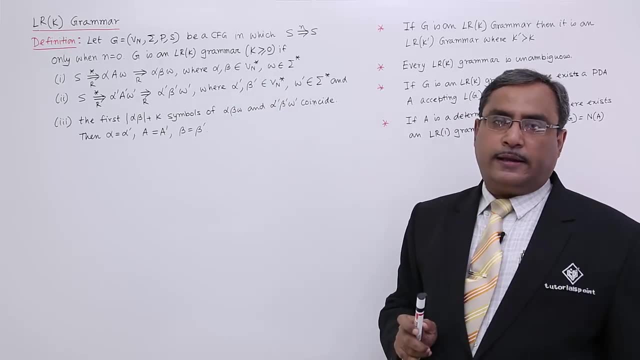 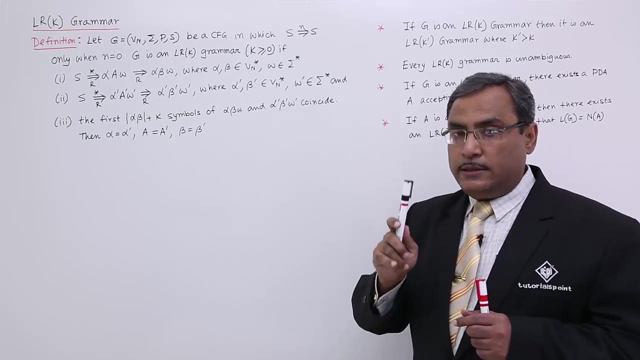 dash, A is equal to A dash and beta is equal to beta dash. So these three conditions are to be satisfied. Then only you can say that this grammar G is LRK grammar. So this is the rigorous definition of LRK grammar. We should have to remember this. and some properties are to